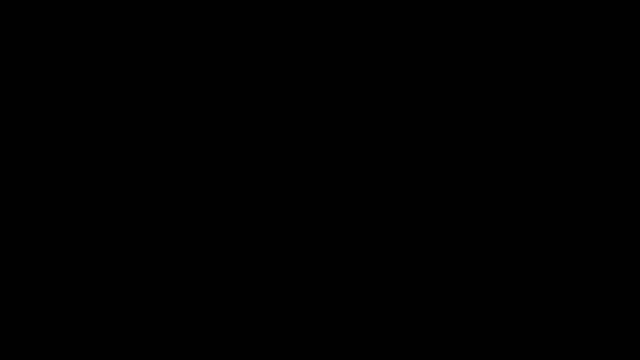 In this video we're going to talk about combustion reactions. In a typical chemistry class, the combustion reactions that you'll encounter usually has to do with some sort of hydrocarbon, and sometimes oxygen might be present. The hydrocarbon always reacts with oxygen in a combustion reaction and the side products are carbon dioxide and water if it's a complete combustion reaction. 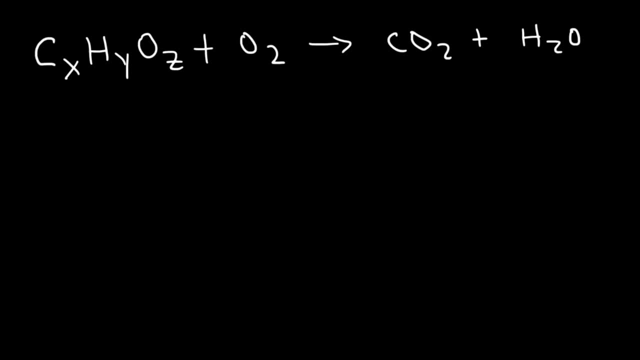 That is, if you react the hydrocarbon with excess oxygen when there's plenty of oxygen available. Now, if you have a limited supply of oxygen, sometimes you might get other products like carbon dioxide, which is a complete combustion reaction. But in a complete combustion you always get CO2 and water, which is typically what you're going to be dealing with. 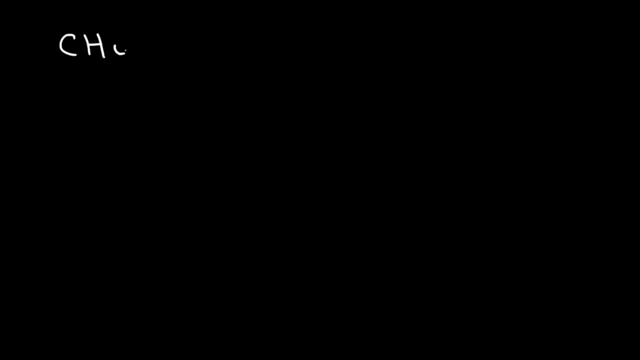 So let's say, if we react methane with excess oxygen, What are the products of the reaction and balance it at the same time? Feel free to pause the video. So for any complete combustion reaction, the products are carbon dioxide and water. Now the best way to know if a combustion reaction is a complete combustion reaction is to use carbon dioxide. 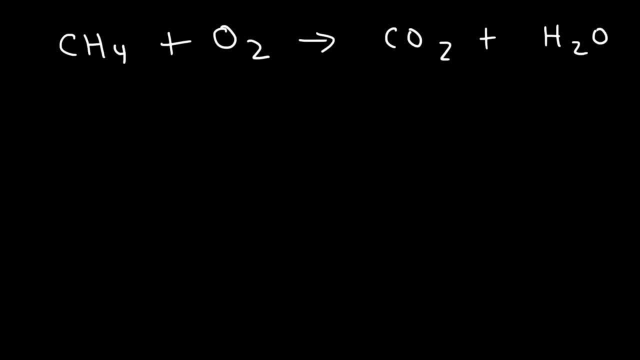 The best way to balance. it is to balance the carbon atoms first. We have one carbon on the left, one carbon on the right, so the carbon atoms are balanced. In the next step, balance the hydrogen atoms. Notice that we have four on the left, two on the right. 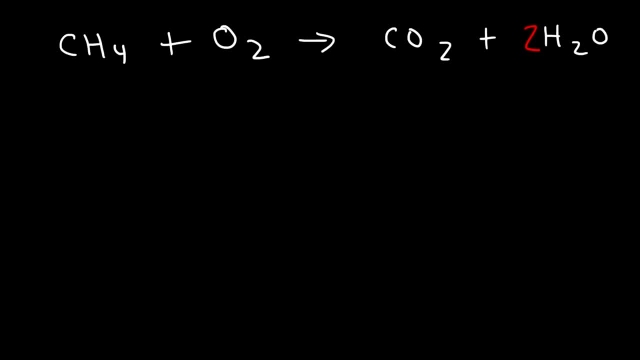 So therefore, to make it equal, we need to put a two in front of H2O. Finally, balance the number of oxygen atoms. On the right side, we have two oxygen atoms. We have two oxygen atoms in carbon dioxide and we have two oxygen atoms in the two water molecules. 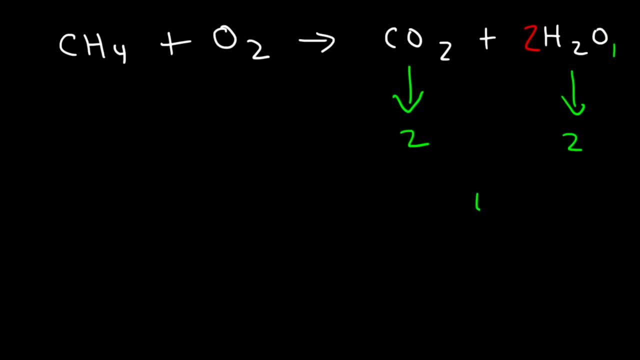 Two times one is two, So we have a total of four oxygen atoms. So therefore we've got to put a two in front of O2 to balance it. Now let's work on another example. Let's react propane with oxygen gas. 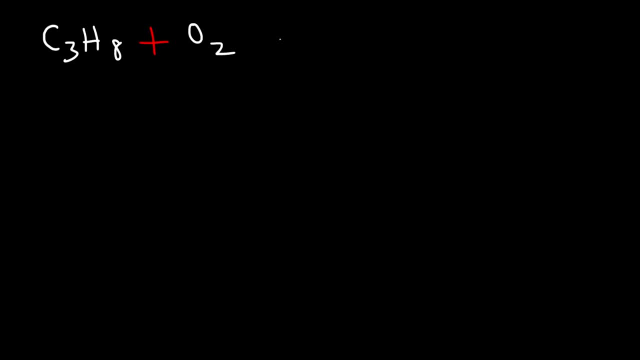 Go ahead and try this problem, Predict the products and balance the reaction. So we know the products is going to be CO2 and H2O. Now, just like before, we're going to balance the carbon atoms first. So notice that we have three carbon atoms on the left and only one on the right. 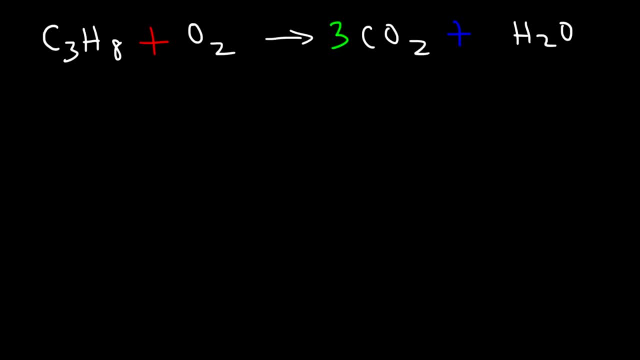 Therefore we've got to put a three in front of CO2.. Next balance, the hydrogen atoms. So we have eight hydrogen atoms on the left, two on the right. Eight divided by two is four, So we've got to put a four in front of H2O. 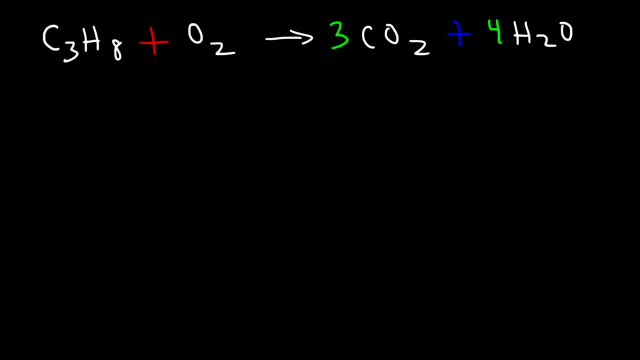 Now we've got to balance the oxygen atoms. What I like to do is count the number of oxygen atoms on the right side and then figure out what number I need to put in front of O2.. So I have four oxygen atoms in the four water molecules, because four times one is four. 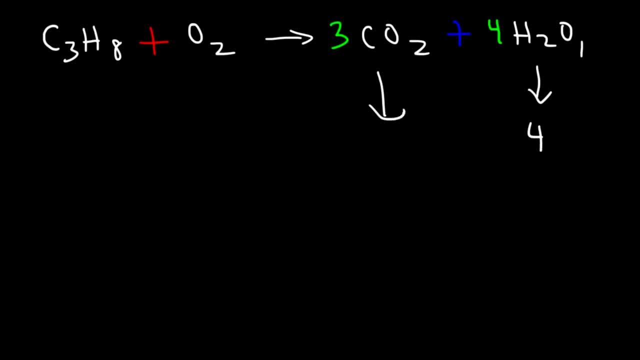 And I have six here, because three times two is six. So basically you multiply the coefficient by the subscript to get the number. So I have a total of four plus six or ten oxygen atoms on the right side. Ten divided by two is five. 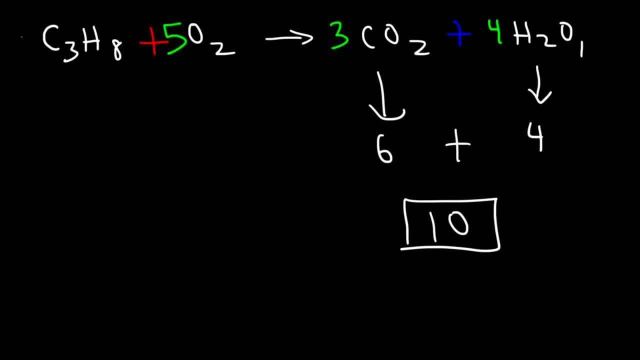 So to balance the reaction, I need to put a five in front of O2.. And so that's it for this particular example. Now let's work on some harder examples. Let's react ethane with oxygen gas. This one might be a little bit more trickier than the last two. 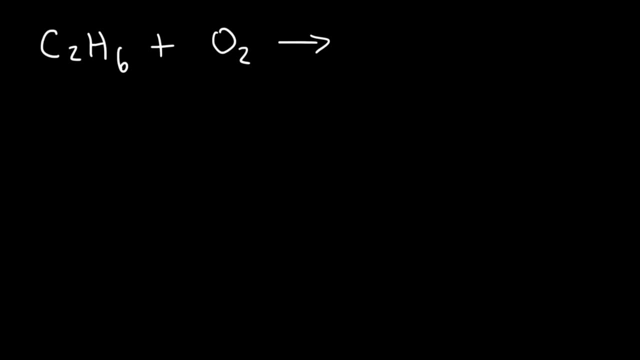 But feel free to pause the video and try it yourself. So the products are CO2 and H2O, So that part is not going to change. Now let's begin by balancing the carbon atoms first. Notice that we have two on the left, one on the right. 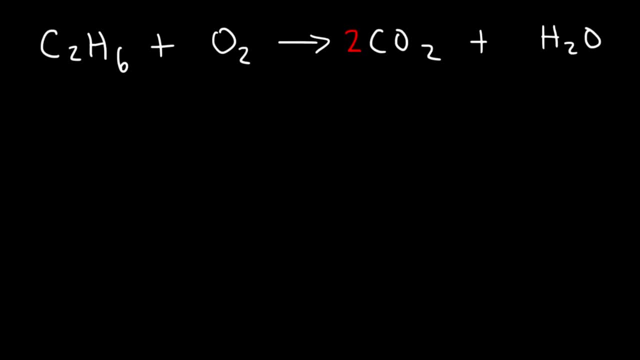 So that means we've got to put a two in front of CO2.. Next let's move on to the hydrogen atoms. We have six on the left, two on the right. Six divided by two is three, So let's put a three in front of H2O. 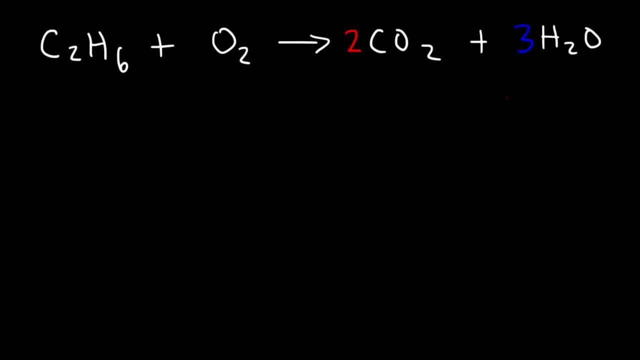 So now we have a total of six hydrogen atoms on both sides. Next let's balance the oxygen atoms. So we have four in the two CO2 molecules, because two times two is four, And in the three water molecules we have three. 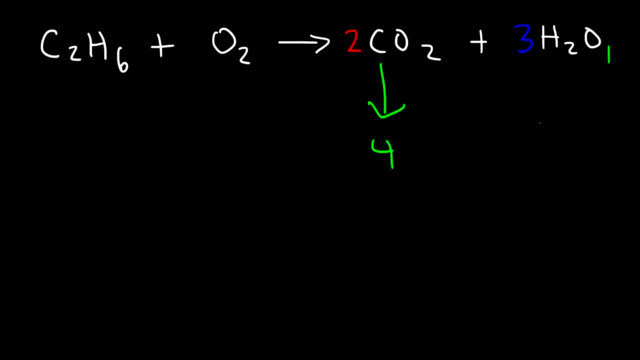 Three times one is three, So we have a total of seven oxygen atoms On the right side. So what number do we need to put in front of O2? What number times two is seven. The opposite of multiplication is division, So you could divide to figure it out. 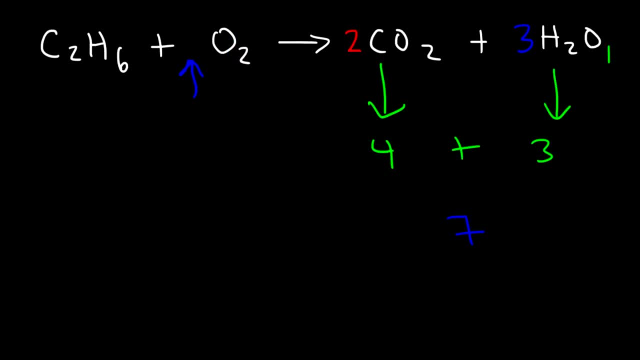 It's going to be seven divided by two, So it's a fraction. The reaction is balanced, but we don't want to leave it like this. We want to get rid of the fractions, So what we're going to do is multiply everything. 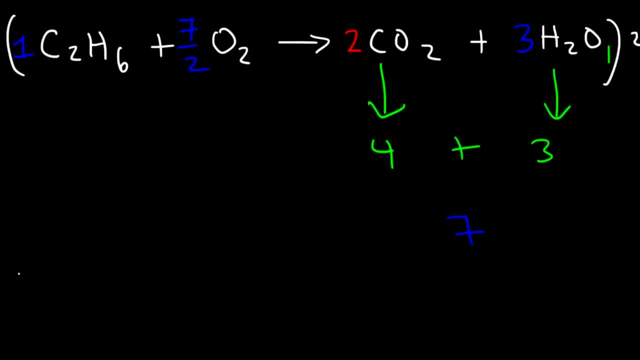 By two All the coefficients, not the subscripts. So it's two ethane molecules. Now two times seven over two, The twos will cancel giving you seven. So this is going to yield seven oxygen molecules. And then two times two is four. 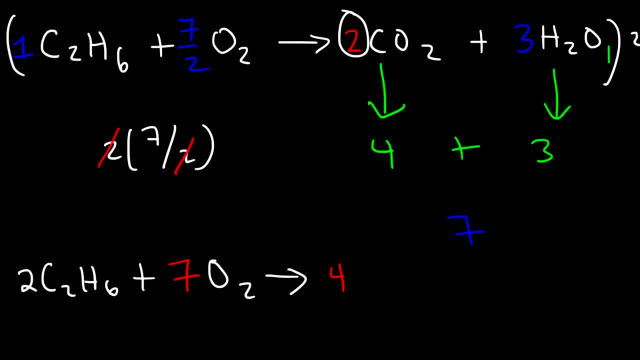 So that's going to be four CO2 molecules, And if we multiply this number by two, it's going to be six H2O molecules. Now the reaction is balanced. Here's a similar example for you to practice on: Go ahead and react with oxygen gas. 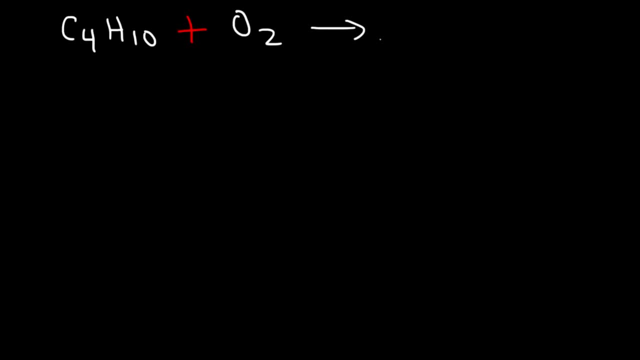 So take a minute and try this example, because the best way to learn is through practice, And that's how you can master this topic. So the products, as always, will be CO2 and H2O, So let's begin by balancing the carbon atoms. 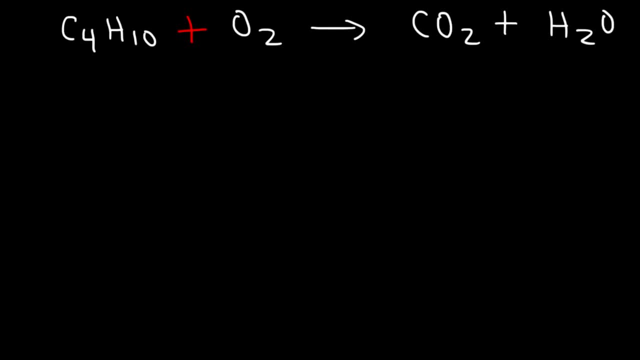 Let's follow the same pattern. Let's follow the same three steps: Balance the carbon atoms first, and then the hydrogen atoms, and then save the oxygen atoms for last, Because oxygen is a pure element on the left side. If you run into a situation where you get an odd number of oxygens on the right side, 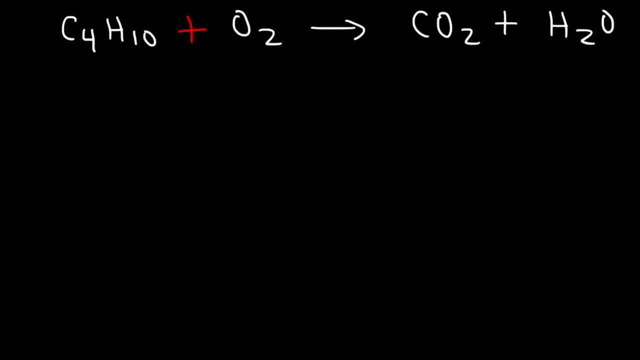 go ahead and balance it as a fraction and then simply multiply everything by two And it's going to work out. So we have four carbon atoms on the left. Therefore, we need to put a four In front of CO2.. Now let's move on to the hydrogen atoms. 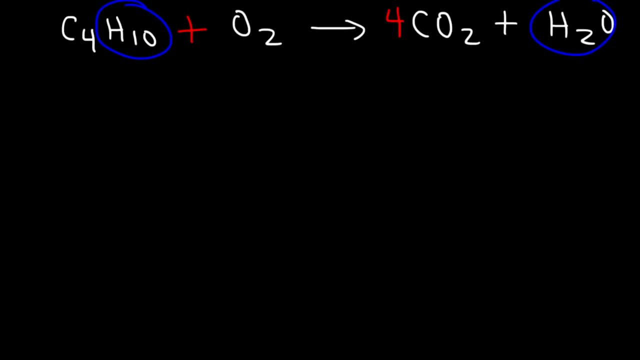 We have ten on the left, two on the right. Ten divided by two is five, So we've got to put a five in front of H2O. Now let's add up the number of oxygen atoms on the right side, So four times two is eight. 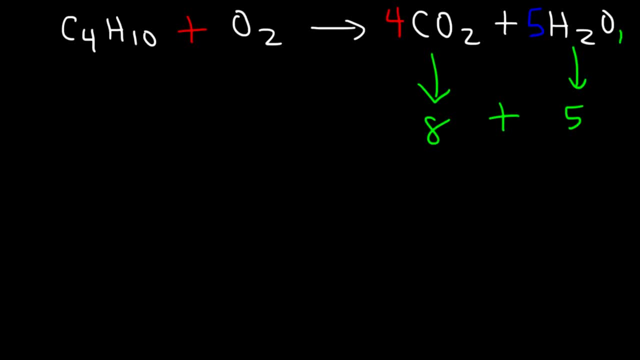 And here we have five times one, which is five. So we have a total of 13 oxygen atoms on the right side. So what number goes in front of O2?? It's going to be 13 divided by two, Or simply 13 over two. 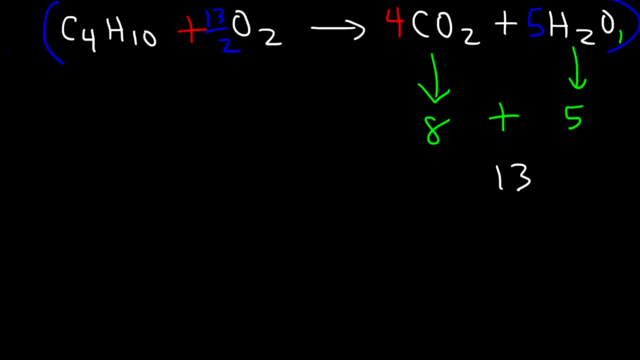 Now the last thing we need to do is multiply everything by two, So we're going to have two butane molecules, C4H10.. And two times 13 over two is just going to be 13.. So we have 13.. 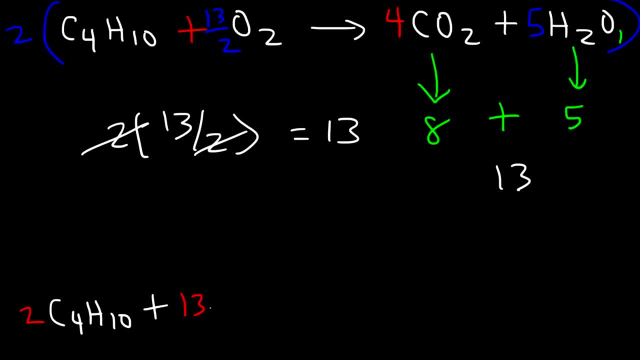 So this is going to be 13 oxygen molecules and that's going to yield 8 carbon dioxide molecules and 10 water molecules. Here's a different example. So let's say, if we have a molecule that contains carbon hydrogen and oxygen, 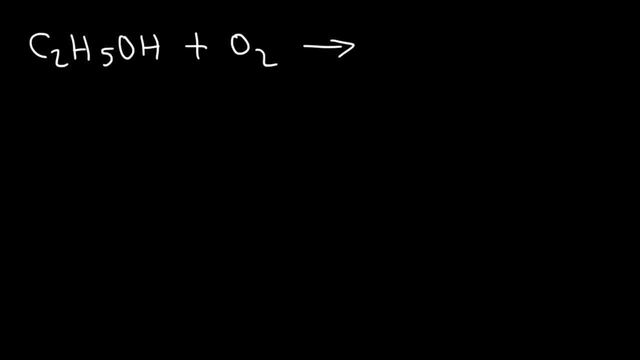 and we're going to react it with oxygen in a combustion reaction. Go ahead and balance the reaction. So the steps for this one is very similar to the previous examples, with one additional step. Let's balance the carbon atoms first. So we got 2 on the left, which means we need to put a 2 in front of CO2.. 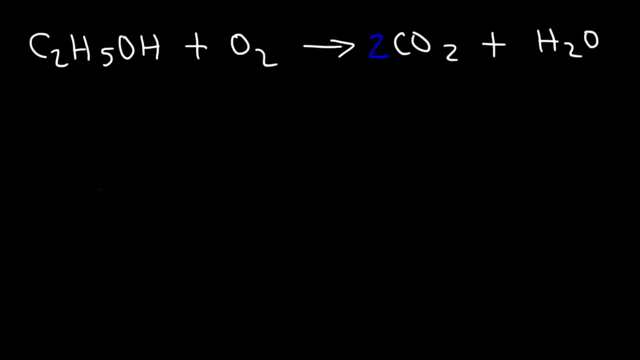 Next let's balance the hydrogen atoms. We have a total of 6 hydrogen atoms on the left. 5 plus 1 is 6. And 6 divided by 2 is 3.. So we need a 3 in front of H2O so that we could have 6 hydrogen atoms on both sides. 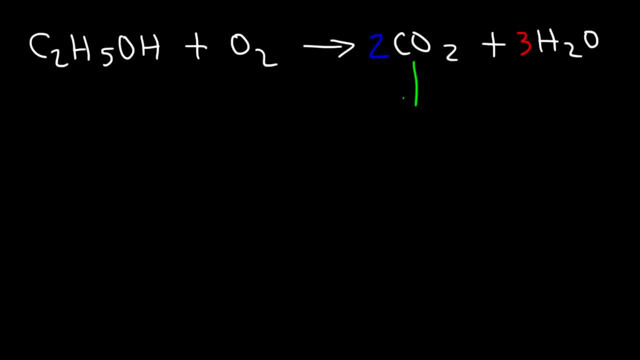 Now let's count the oxygen atoms on the right. 2 times 2 is 4, so we have 4 oxygen atoms in the 2 CO2 molecules and we have 3 in the 3 water molecules. 4 plus 3 is 7.. 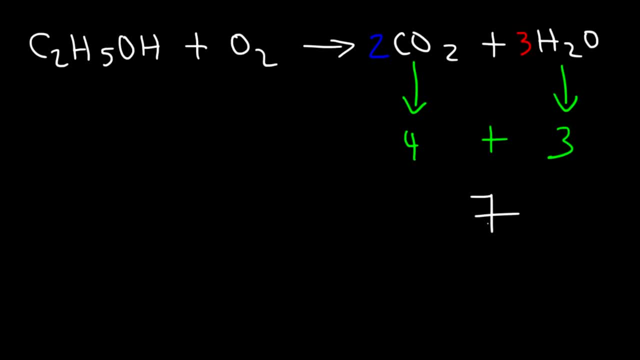 Now we have an odd number, but for this example it's not a problem, because we already have 1 oxygen atom. We just need to put a 2 in front of CO2.. And to get to 7, we need 6, because 1 plus 6 is 7, and 6 divided by 2 is 3.. 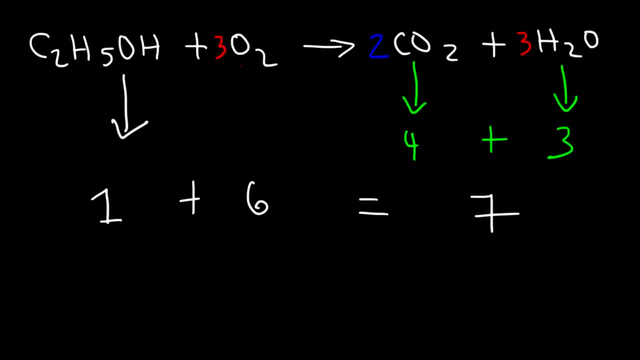 So we need a 3 in front of O2.. So notice that we have 2 carbon atoms on both sides. We have a total of 6 hydrogen atoms on both sides. 5 plus 1 is 6.. And the number of oxygen atoms on both sides is 6.. 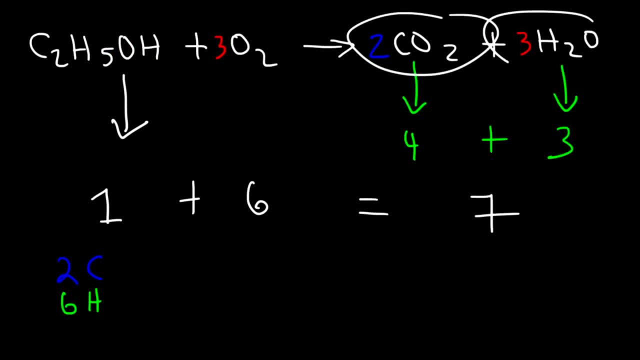 So we have a total of 6 hydrogen atoms on both sides. 5 plus 1 is 6.. And the number of oxygen atoms on both sides is 7.. Here we have 4,, that's 3.. And here, 3 times 2 is 6, plus 1, that's 7.. 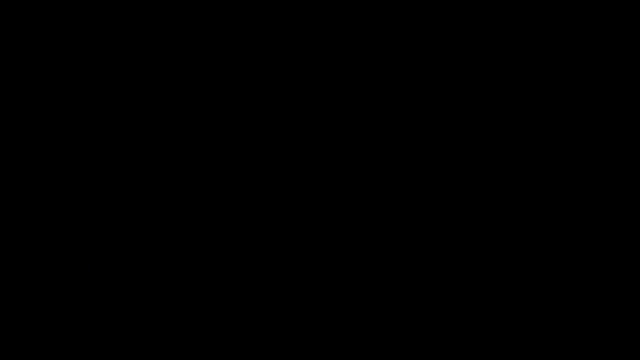 So everything is balanced. So this is going to be the last example of this video. So in this example we have propanol and we're going to react it with oxygen to produce carbon dioxide and water. So let's follow the same examples. 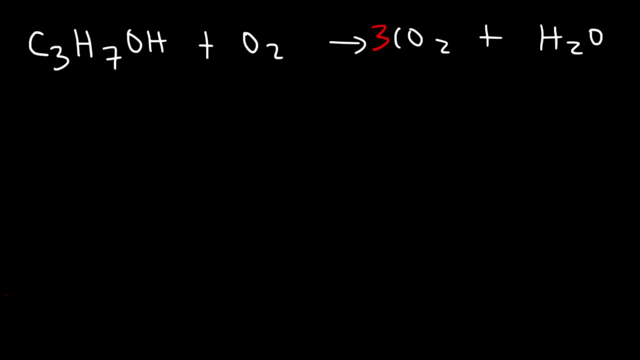 We have 3 carbon atoms on the left, So we're going to put a 3 in front of CO2.. Now we have a total of 8 hydrogen atoms. 7 plus 1 is 8.. And 8 divided by 2 is 4.. 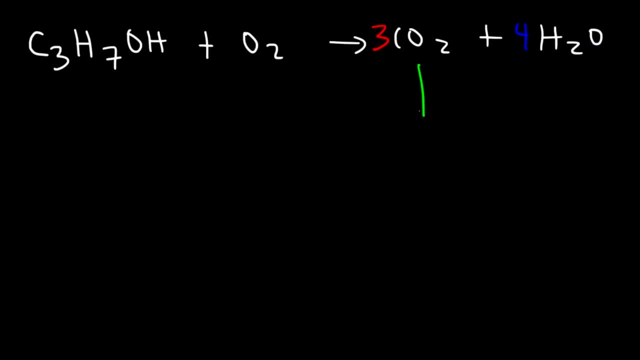 So we're going to put a 4 in front of H2O, And then here we have 6 oxygens. that's 3 times 2.. That's a terrible looking 6.. And here we have 4 oxygens in the 4 water molecules. 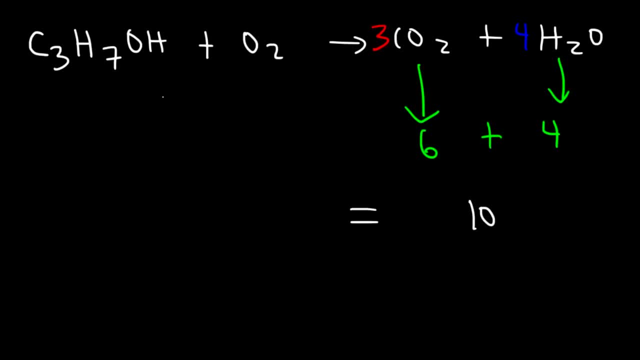 Now 6 plus 4 is 10.. Now we have 1 oxygen in propanol. So 1 plus 9 is 10.. Therefore we need to get 9 oxygens in the O2 molecules. So here we're going to get a fraction. 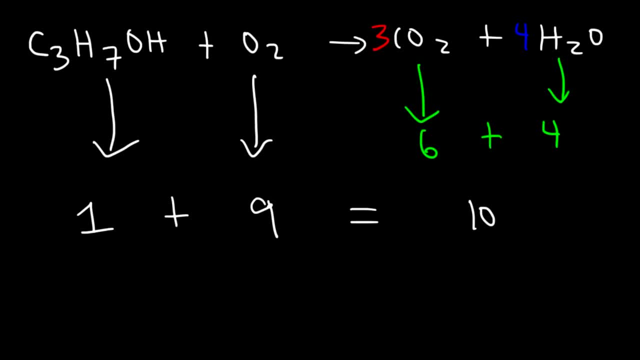 9 divided by 2 is 9 over 2.. So what we need to do is multiply everything by 2 to get rid of that fraction. So it's going to be 2 propanol molecules plus 2 times 9 over 2..